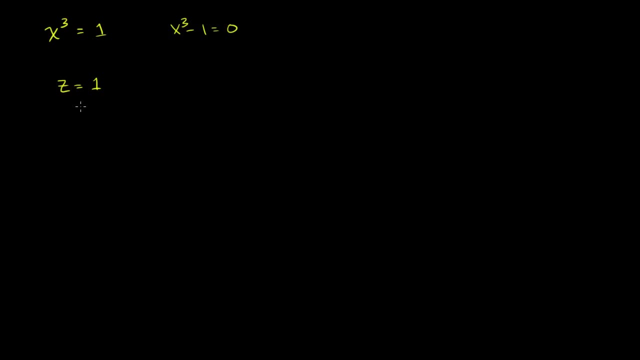 1 is a complex number. It's a real number, Real number, All real numbers are also complex numbers. They're a subset, They're in the complex plane, They just don't have an imaginary part. So let's draw this on an Argand diagram. 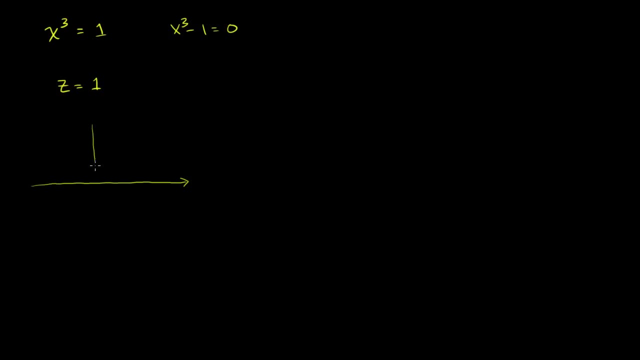 So that's my real axis, This is my imaginary axis, And so this is the real, This is the imaginary. And if I wanted to represent, z equals 1, it only has a real part, So let me just draw 1 all around. 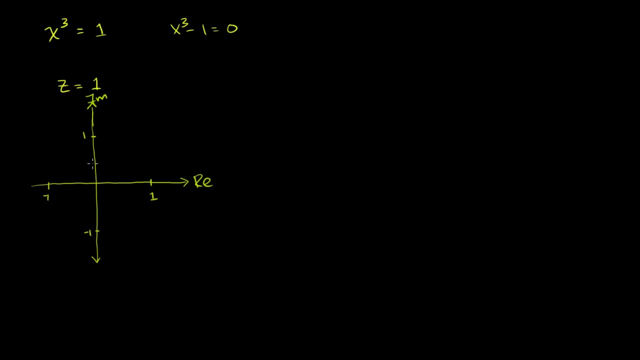 Negative 1, negative 1.. z looks like this. z would look like that: A position vector that just goes to 1, 0.. One way to view it- this is the same thing- is equal to 1 plus 0i. 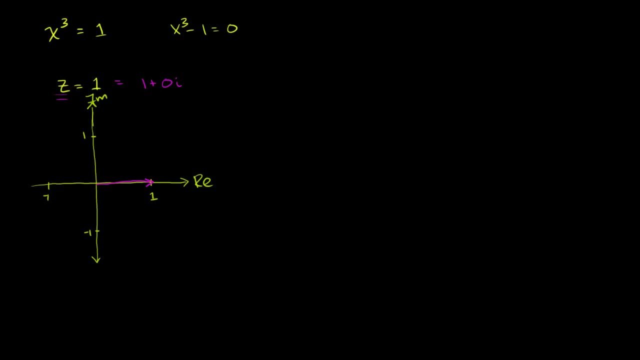 Now let's put this in exponential form. Well, its magnitude is pretty straightforward: 1 plus 0i. The magnitude of z is just the length of this vector, or it's the absolute value of 1.. That's just going to be 1.. 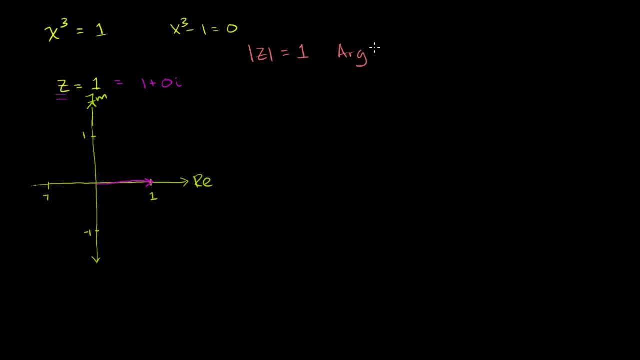 Now, what's the argument of z? What's the angle that this vector makes with the positive real axis? What's on the positive real axis? It's a real number, So it has no angle, So the Arg of z is 0.. 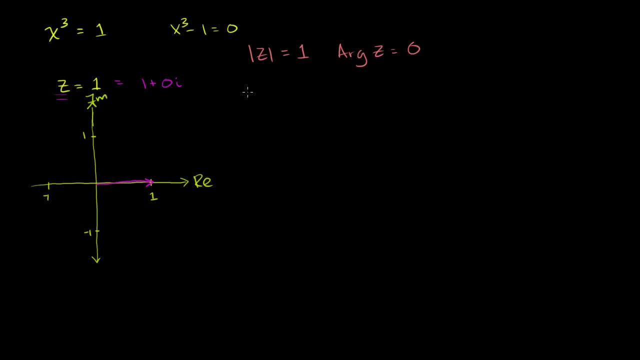 So that might not be too interesting. so far, We just wrote it. We just figured out that 1 could be equal to. 1 is equal to 1 times e to the 0i, And this is kind of obvious. e to the 0, this is going to be 0. 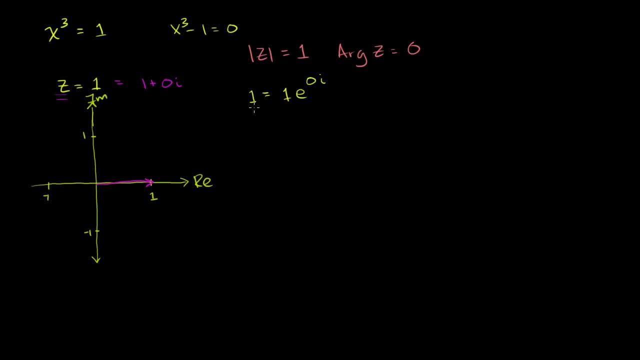 0 times i is 0.. e to the 0 is going to be 1 times 1 is equal to 1.. Not a big deal there. But what is neat is that this argument. you could view it as 0 radians, or you could go all the way. 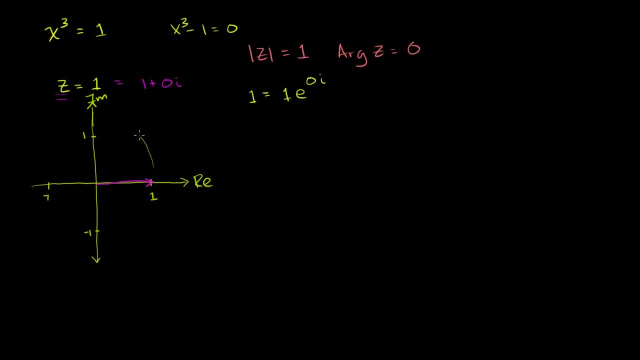 around and add 2 pi to it and get to the same point. You can go all the way around, All the way around and add 2 pi and get to the same point. So the argument of our complex number or of the number 1, 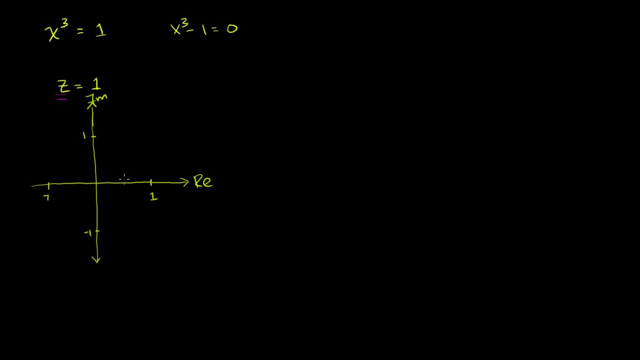 z looks like this. z would look like that: a position vector that just goes to 1, 0.. One way to view it- this is the same thing- is equal to 1 plus 1 plus 0i. Now let's put this in exponential form. 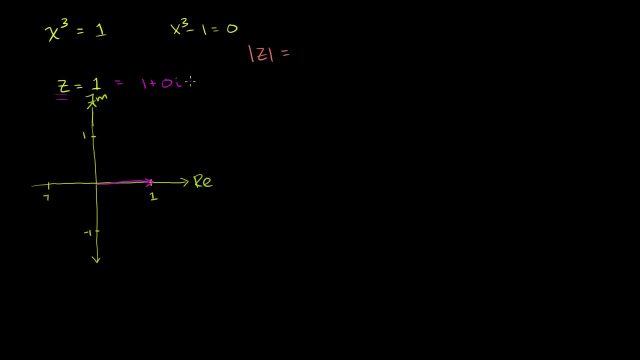 Well, its magnitude is pretty straightforward. The magnitude of z is just the length of this vector, or it's the absolute value of 1.. And that's just going to be 1.. Now, what's the argument of z? What's the angle that this vector makes? 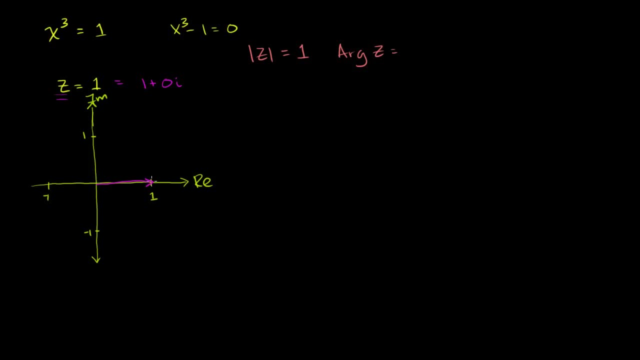 with the positive real axis. What's on the positive real axis? It's a real number, So it has no angle. So the Arg of z is 0. So that might not be too interesting. so far We just wrote. We just figured out that 1 could be equal to 1. 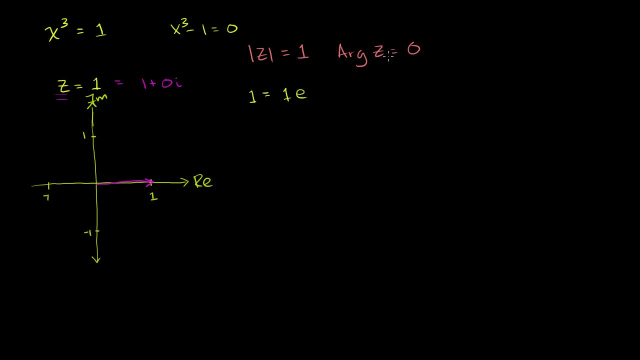 is equal to 1 times e to the 0i, And this is kind of obvious. e to the 0,, this is going to be 0.. 0 times i is 0.. e to the 0 is going to be 1 times 1 is equal to 1.. 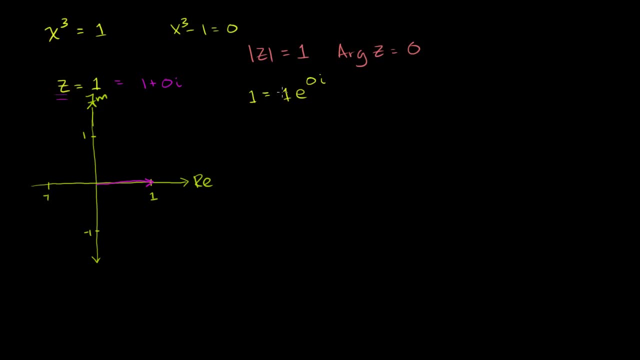 Not a big deal there. But what is neat is that this argument- you could view it as 0 radians, or you could go all the way around and add 2 pi to it and get to the same point. You can go all the way. 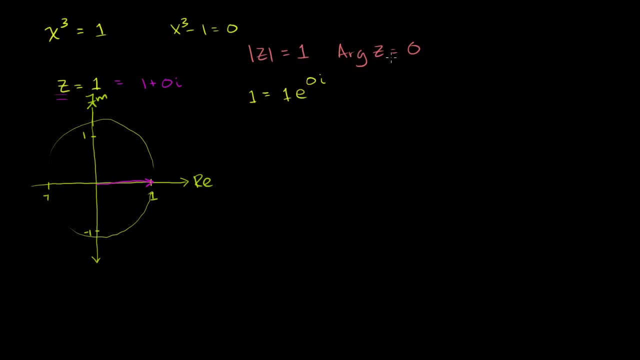 You can go all the way around and add 2 pi and get to the same point. So the argument of our complex number or of the number 1 really could also be an angle of 2 pi or an angle of 4 pi. 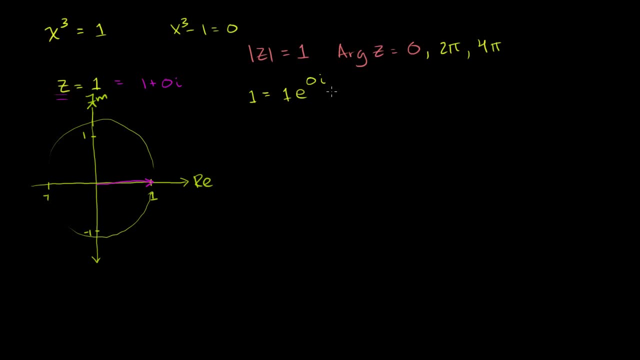 or an angle of 6 pi or an angle of 8 pi. So we can write 1 as 1 times e I won't write the 1 anymore. 1 times e to the 2 pi i or 1 times e to the 4.. 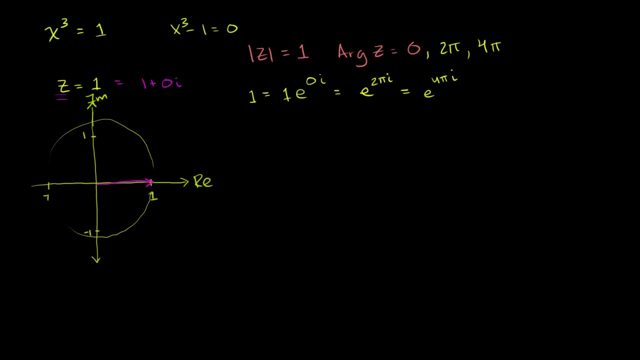 And the reason why this is interesting is in this equation. this equation right here can be written in multiple ways. It can be written as: x to the third is equal to 1.. It could be written as: x to the third is equal to e to the 2 pi. 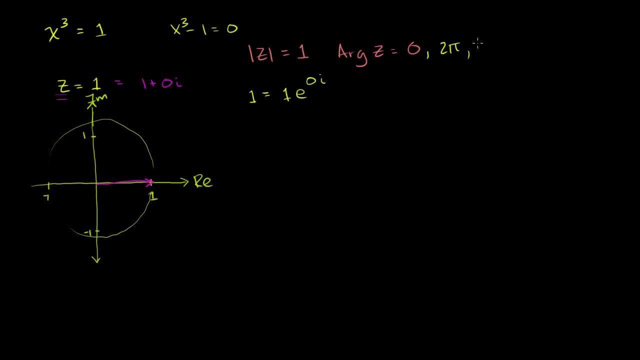 really could also be an angle of 2 pi or an angle of 4 pi, or an angle of 6 pi or an angle of 8 pi. So we can write 1 as 1 times e I won't write the 1 anymore. 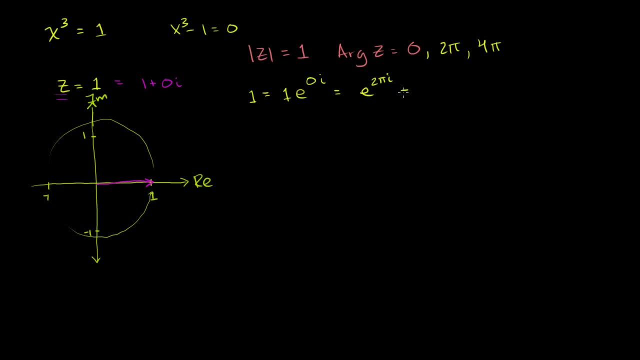 1 times e to the 2 pi i or 1 times e to the 4. To the 4 pi i. And the reason why this is interesting is in this equation. this equation right here can be written in multiple ways. 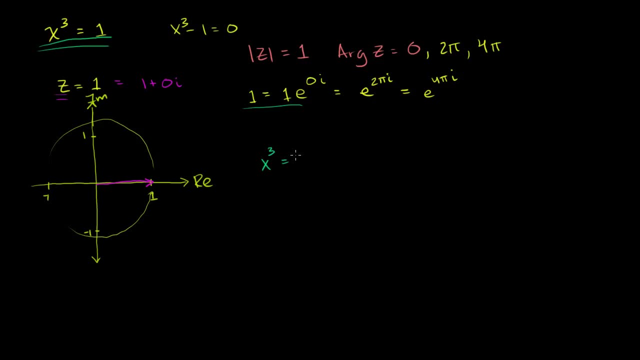 It can be written as: x to the 3rd is equal to 1.. It could be written as: x to the 3rd is equal to e to the 2 pi i. Or it can be written as x to the 3rd. 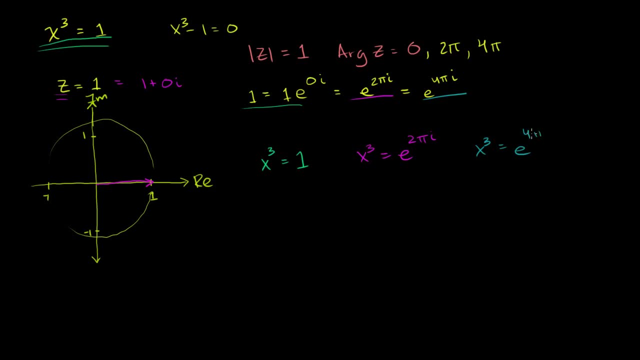 is equal to e to the 4 pi i, And this is interesting And we're going to see this in a second. Let's take both sides of all these equations to the 1 third, power to solve for x. So to the 1 third. we're going to take that to the 1 third. 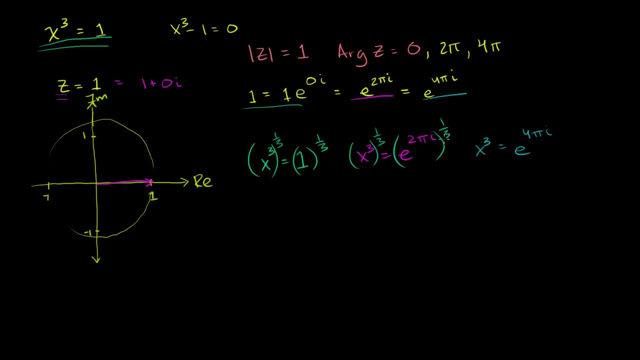 We're going to do that same thing over here. We're just taking everything to the 1 third power to solve for the x's in each of these equations To the 1 third power. So this first equation over here becomes: x is equal to 1 to the 1 third power. 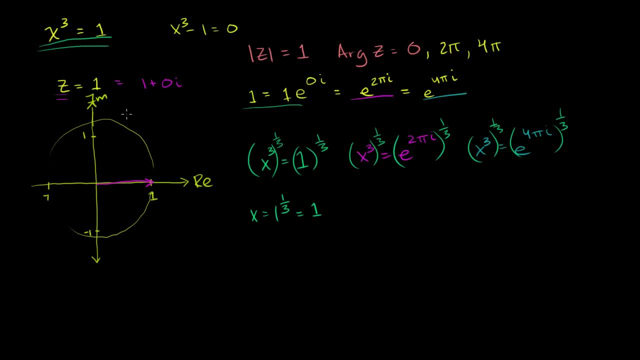 which is just equal to 1.. Now, what's the second equation become? This second equation: x is equal to e to the. well, this is going to be the 2 pi over 3 i power. e to the 2 pi over 3 i power. 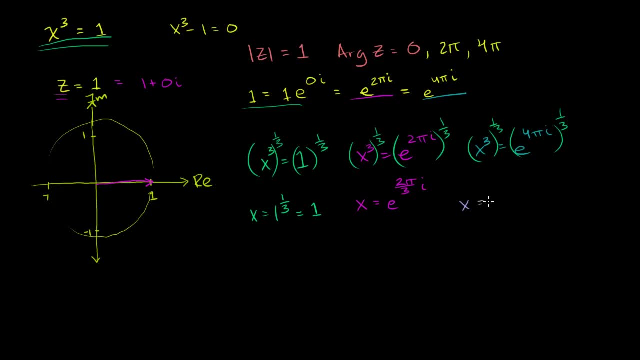 And then this equation over here is going to be: so: x is going to be equal to, obviously, the 3 to the 1 third. that just becomes x to the 1. x is going to let me do that same blue. 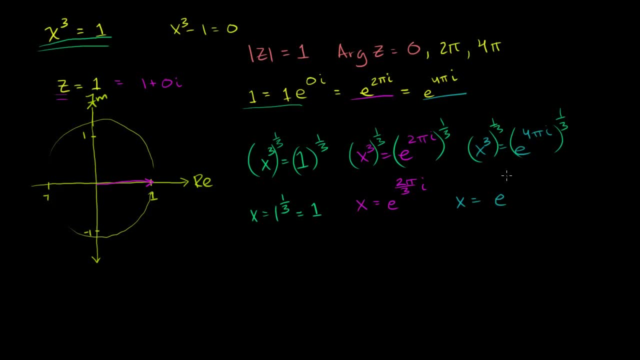 x over here is going to be equal to e, to the 4 pi Over 3, the 4 pi over 3, i. So let's think about this for a little bit. What is this So we could so immediately? what's the argument here? 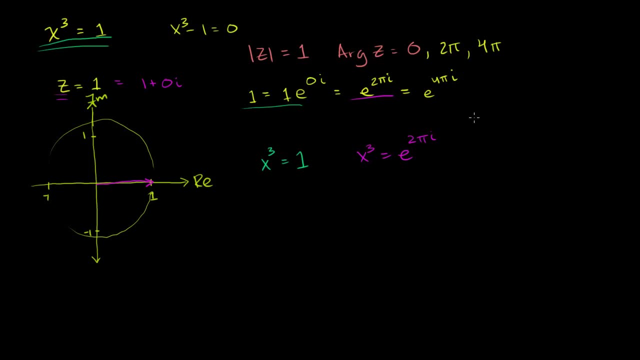 i, or it could be written as: x to the third is equal to e to the 4, pi i- And this is interesting, We're going to see this in a second. Let's take both sides of all these equations to the 1 third power to solve for x. 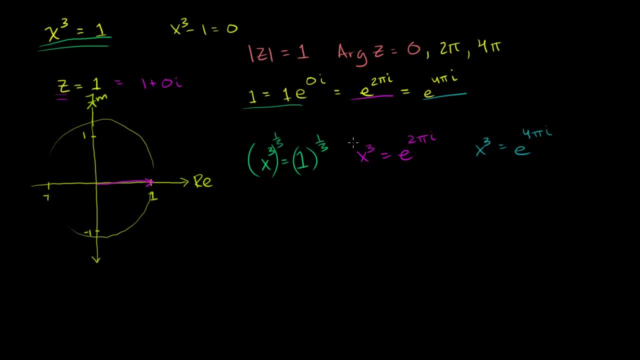 So to the 1 third. we're going to take that to the 1 third. We're going to do that same thing over here. We're just taking everything to the 1 third, power to solve for the x's in each of these equations. 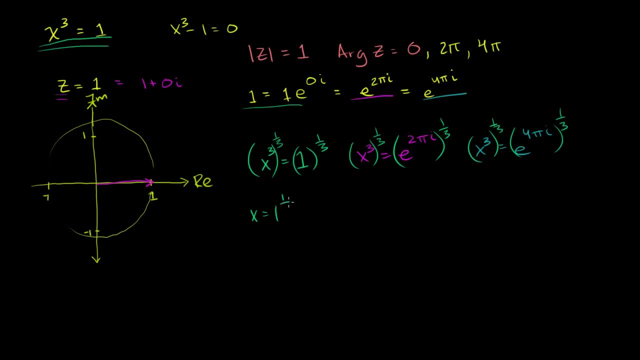 So this first equation over here becomes: x is equal to 1 to the 1 third power, which is just equal to 1.. Now what's the second equation become? This second equation: x is equal to e to the 2 pi over 3 i power. 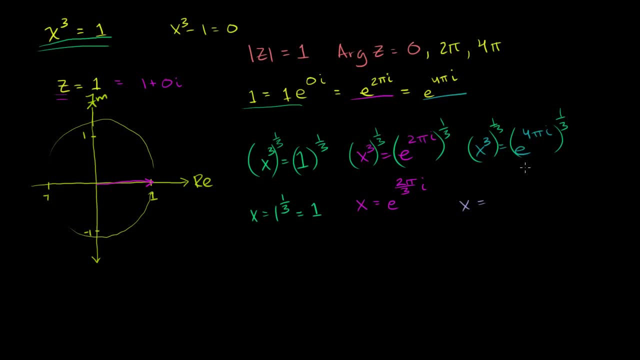 Then this equation over here is going to be: So: x is going to be equal to, obviously, the 3 to the 1 third. That just becomes x to the 1.. Let me do that same blue x over here is going to be equal to e to the 4 pi. 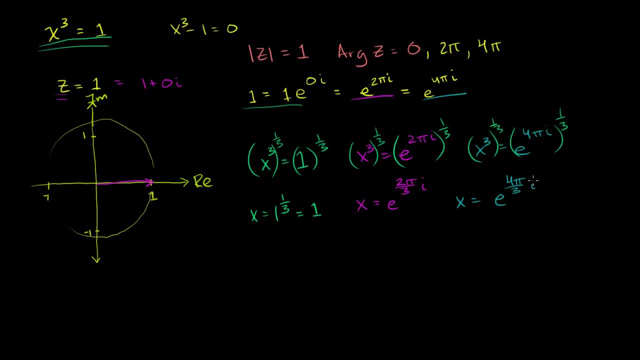 over 3, i power. Well, it's just going to be that one here over 3, the 4 pi over 3i. So let's think about this for a little bit. What is this So immediately? what's the argument here? 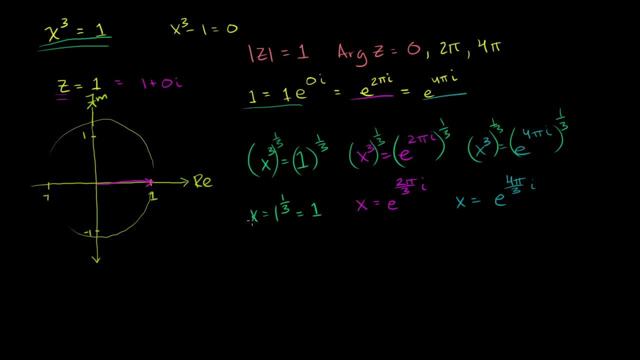 So let me write: These are three different roots. Let me call this x1,, x2, and x3.. So these are three different numbers. One of the roots is 1.. That's pretty clear over here. 1 is one of the cube roots of itself. 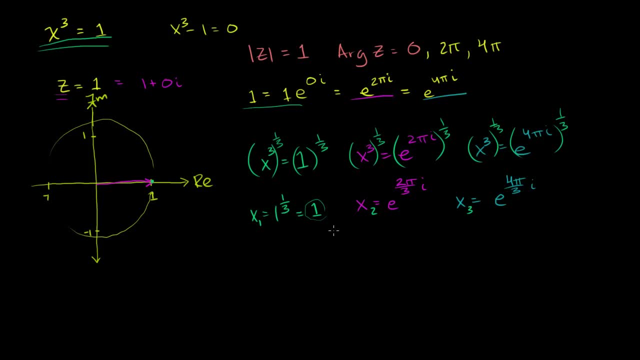 But these are other numbers And these are going to be complex numbers. So let's visualize these numbers a little bit. So what is the argument? So, for all of these? so the magnitude of x2 is still clearly 1. It's the coefficient out in front of the e. 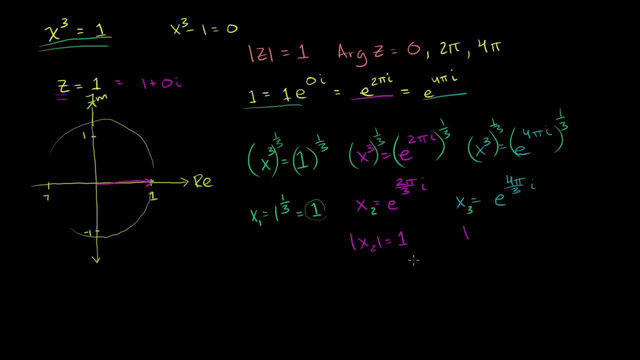 It's clearly 1.. The magnitude of x3, let me do that same color. The magnitude of x3 is also clearly going to be 1.. But what is the argument of x2?? What is phi? What is the argument? 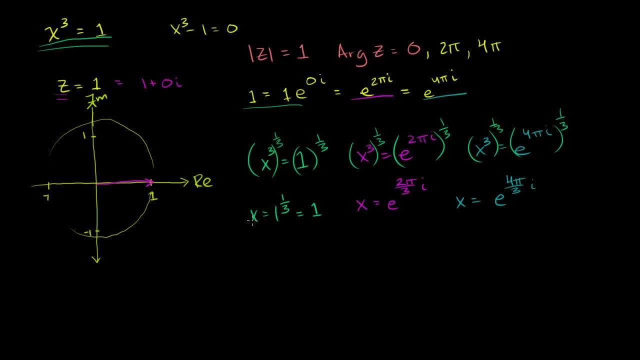 So let me write: these are three different roots. Let me call this x1,, x2, and x3.. So these are three different numbers. One of the roots is 1.. That's pretty clear over here. One is one of the cube roots of itself. 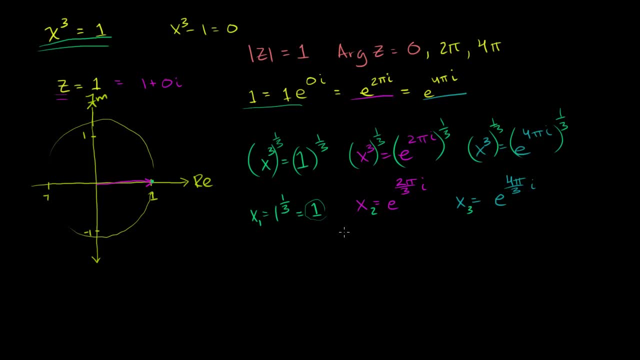 But these are other numbers And these are going to be complex numbers. So let's visualize these numbers a little bit. So what is the argument? So, for all of these? so the magnitude of x2 is still clearly 1. It's the coefficient out in front of the e. 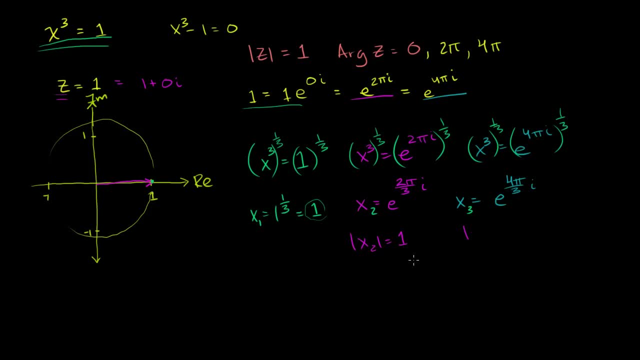 It's clearly 1.. The magnitude of x3, let me do that same color. The magnitude of x3 is also clearly going to be 1.. But what is the argument of x2?? What is phi? What is the argument? 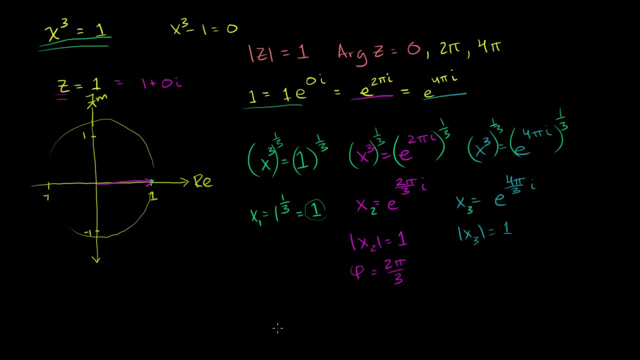 Well, it's 2 pi over 3.. It's 2 pi over 3.. So how would we draw x2?? So the angle is 2 pi over 3.. It's easier for me to visualize in degrees. So 2 pi is 360 degrees. 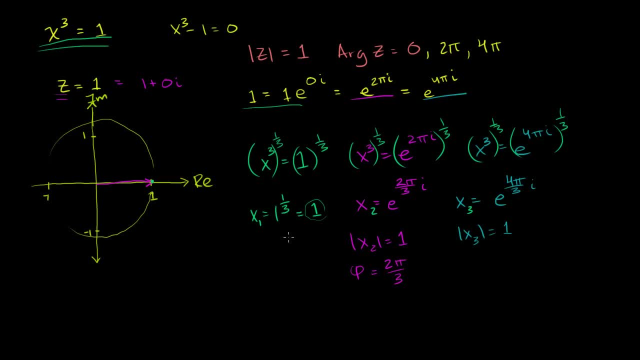 360 degrees divided by 3 is 120 degrees, So this is going to be 120 degrees is 60 short of, so it's going to look like this. It's going to look like this. Just like this, Just like this. 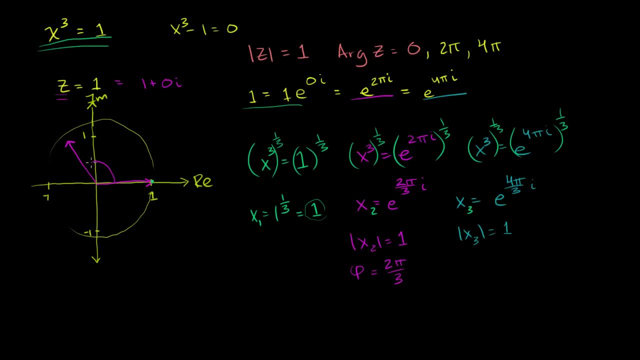 Just like this. So this angle right here, its argument is going to be 120 degrees, which is the same thing as 2 pi over 3. And it's going to have the exact same length. Let me do the same color. 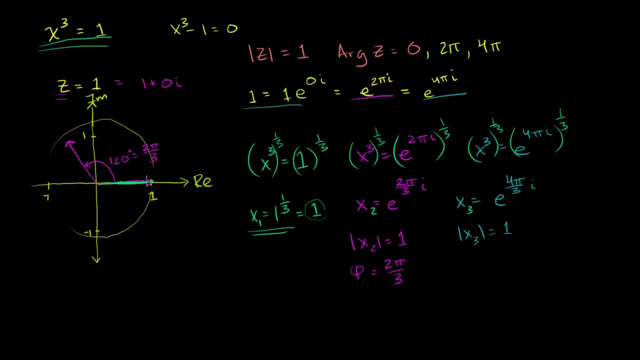 So this is x1.. So that is this green color right over here. x2 is this magenta one right over here, And they all have the same magnitude. So we really just rotated. We rotated 120 degrees, And what about x3?? 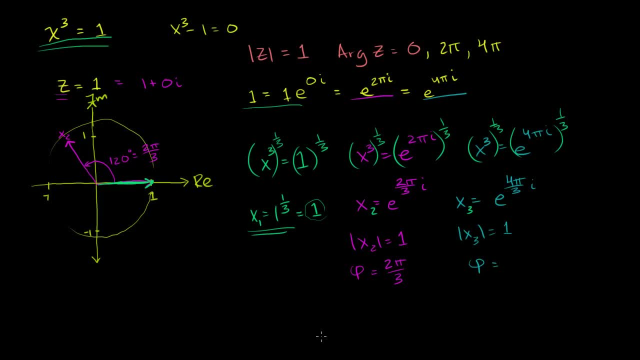 What's its argument? What's x3's argument? Its argument is 4 pi over 3.. That's the same thing as 720 degrees over 3, if we were to put it into degrees, And so 3 goes into 720.. 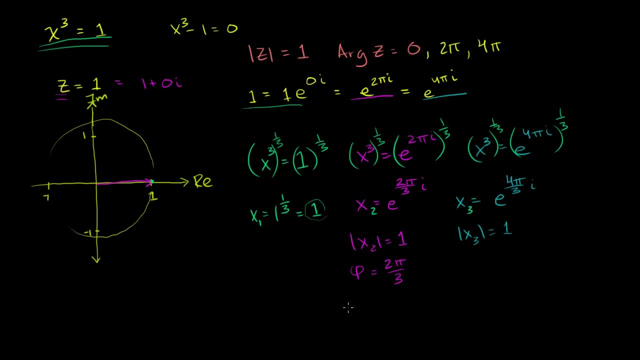 Well, it's 2 pi over 3.. It's 2 pi over 3.. So how would we draw x2?? So the angle is 2 pi over 3.. It's easier for me to visualize in degrees. So 2 pi is 360 degrees. 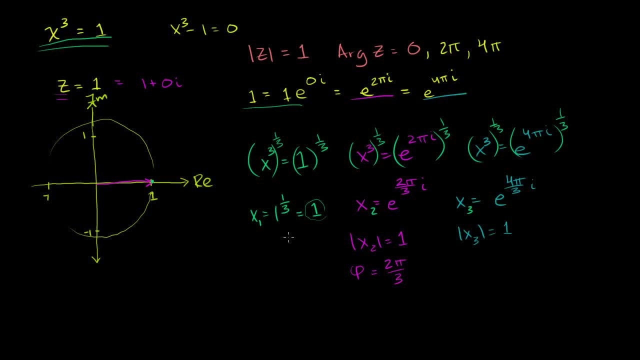 360 degrees divided by 3 is 120 degrees, So this is going to be 120 degrees is 60 short of, so it's going to look like this. It's going to look like this. Just like this, Just like this. 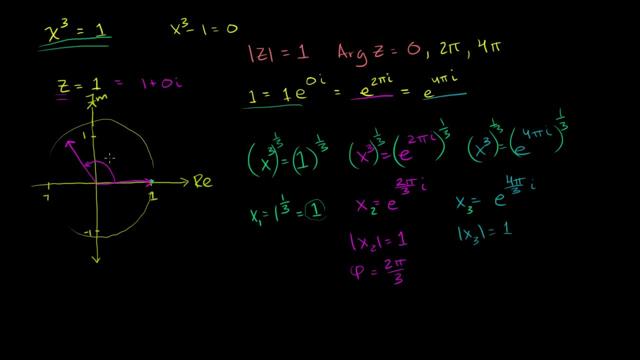 So this angle right here, its argument is going to be 120 degrees, which is the same thing as 2 pi over 3. And it's going to have the exact same length. Let me do the same color. So this is x1.. 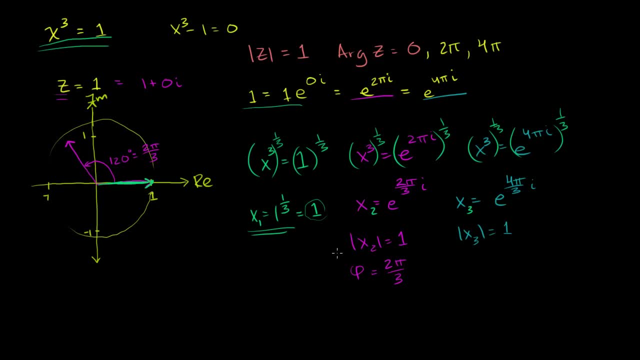 So that is this green color right over here, x2 is this magenta one right over here, And they all have the same magnitude. So we really just rotated. We rotated 120 degrees. And what about x3?? What's its argument? 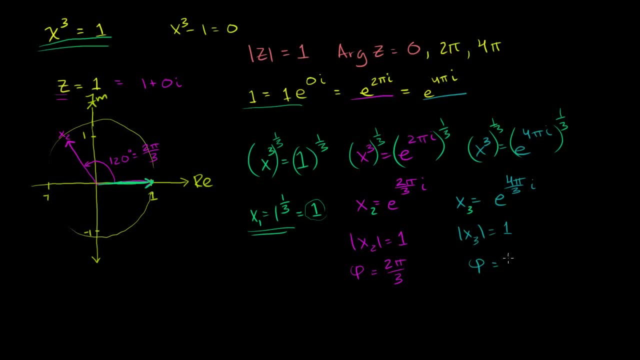 What's x3's argument? Its argument is 4 pi over 3.. That's the same thing as 720 degrees over 3, if we were to put it into degrees, And so 3 goes into 720.. 3 goes into 720.. 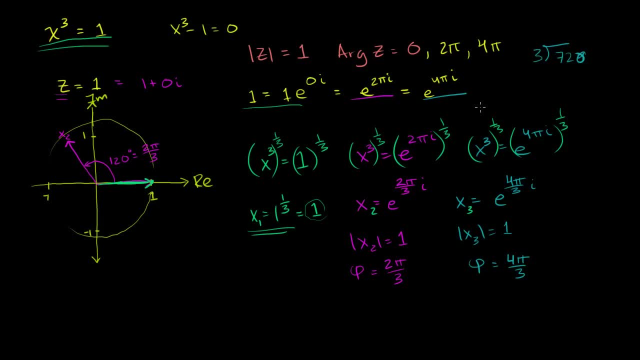 3 goes into 720.. What is it? 240? 720. 240.. Right, I should have known that. So 240 degrees, We're going to go 180 degrees And then go another 60 degrees, So it's going to be right over here. 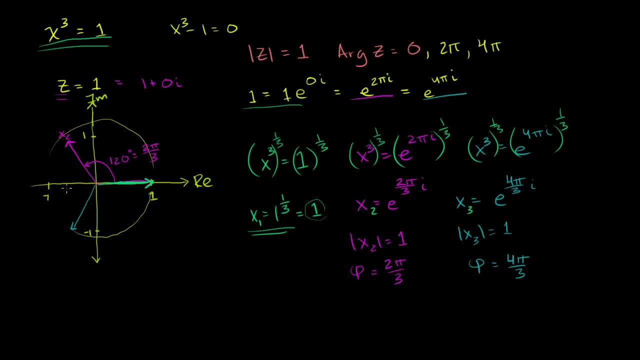 Let me draw it like this: It's going to be right over here, So this is going to be that angle. right over there is 4 pi over 3 radians, which is equal to 240 degrees, And once again it has the same magnitude. 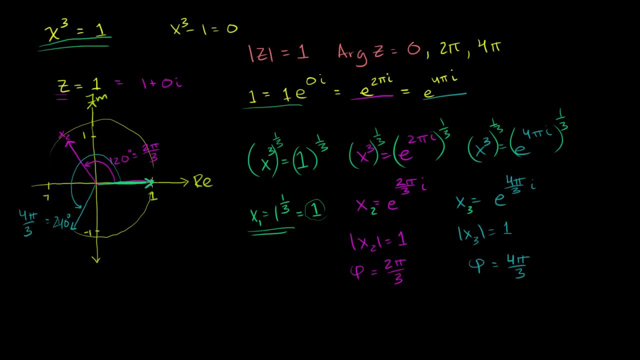 So what we just saw is, when I take the cube roots of this real number, I'm essentially taking the entire- I guess we could call it the entire circle, or the entire 360 degrees, or the entire 2 pi radians, and I'm dividing it into angle, into 3, essentially. 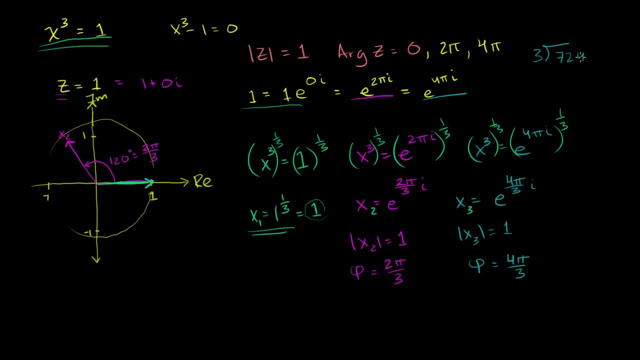 3 goes into 720.. 3 goes into 720.. What is it? 240? 720. 240.. Right, I should have known that. So 240 degrees, We're going to go 180 degrees and then go another 60 degrees. 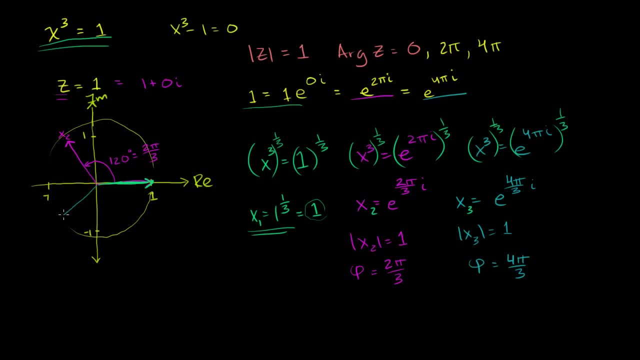 So it's going to be right over here. It's going to be right over here. Let me draw it like this: It's going to be right over here, So this is going to be that angle: right over there is 4 pi over 3 radians, which is equal to 240 degrees. 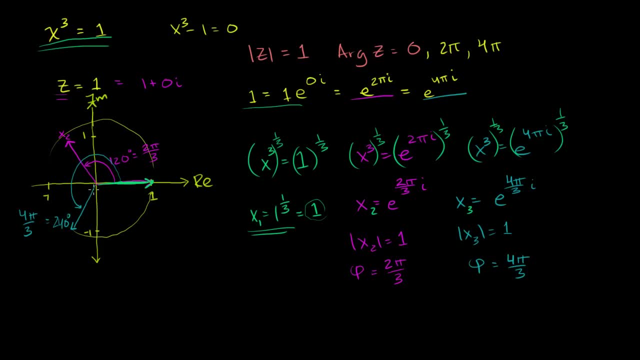 And once again it has the same magnitude. So what we just saw- Because when I take the cube roots of this real number, I'm essentially taking the entire, I guess we could call it the entire circle, or the entire 360 degrees, or the entire 2 pi radians- 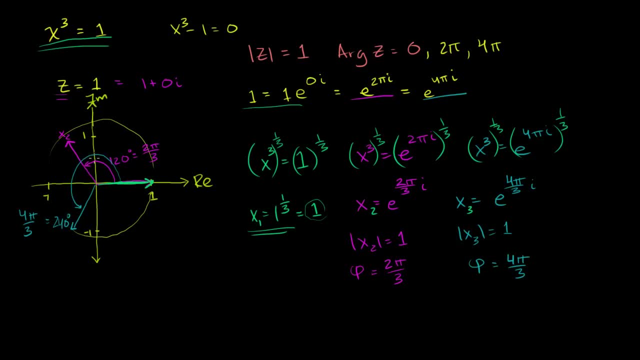 and I'm dividing it into angle, into 3. essentially This is 1 third. Then we have another 120 degrees, And then we have another 120 degrees, And so you kind of see the pattern of where all of the roots are. 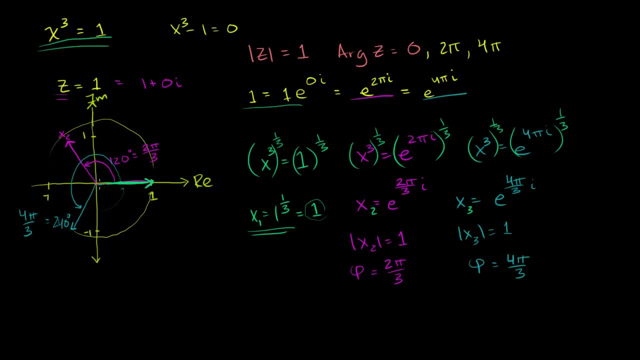 And in case you're still not satisfied, you're like: well, you said you would find complex roots. Yeah, You know I'm not used to this or this as actually being complex numbers. I actually want it to be in the form a plus bi. 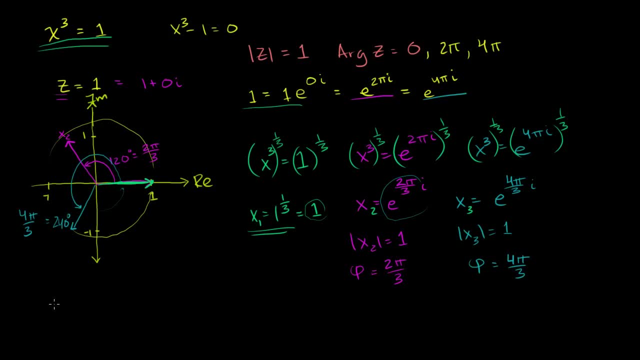 We can easily figure it out from this right over here. So x2 is going to be equal to the cosine of 2 pi over 3, plus i times the sine of 2 pi over 3.. And if you look at this over here, 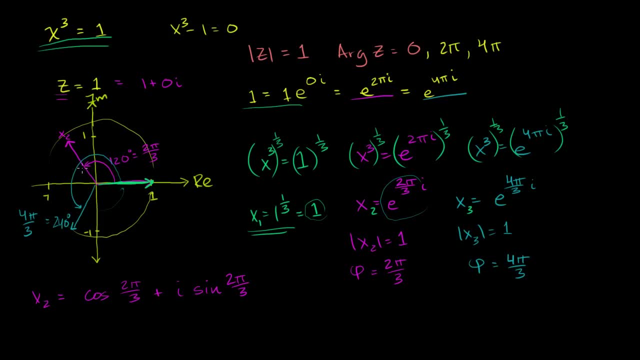 we can figure out what those things are going to be. This is the angle right over here. If this angle right over here is 60 degrees, which it is because this up here is 30 degrees, and the hypotenuse or the length is 1,, 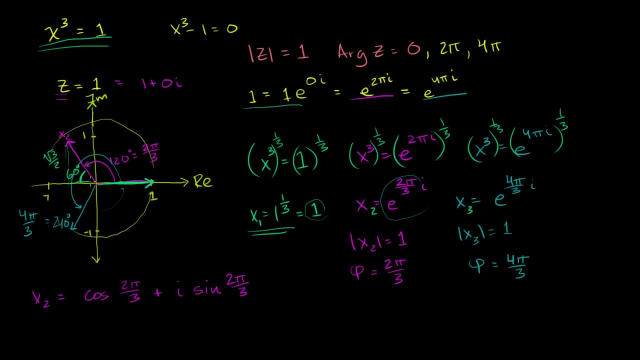 then this over here is square root of 3 over 2. And at this distance right over here is negative 1 half. So x2 is going to be equal to cosine of 2. pi over 3 is negative 1. 1 half. 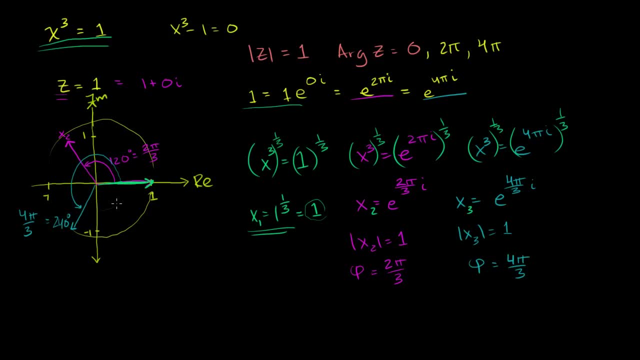 This is 1 third. Then we have another 120 degrees, And then we have another 120 degrees, And so you kind of see the pattern of where all of the roots are. And in case you're still not satisfied, you're just like: well, you said you would find complex roots. 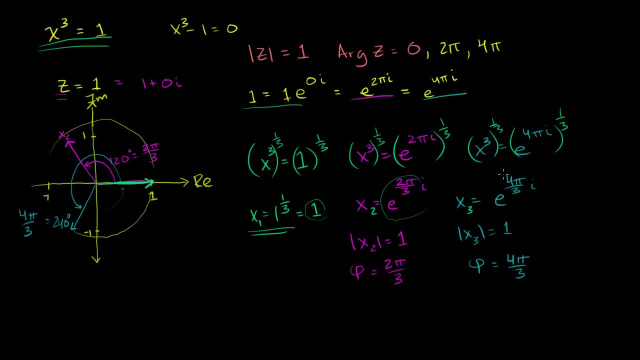 Yeah, You know I'm not used to this or this. So this is actually being complex numbers. I actually want it to be in the form a plus bi. We can easily figure it out from this right over here. So x2 is going to be equal to the cosine of 2 pi over 3. 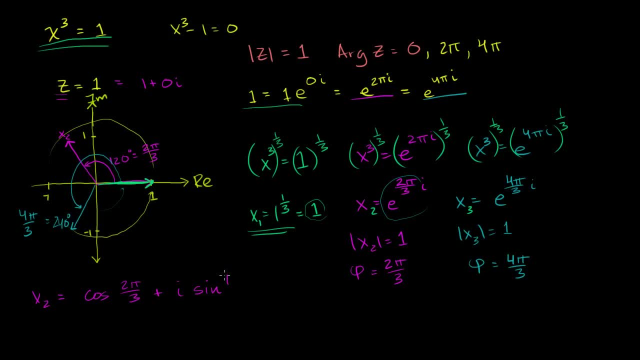 plus, i times the sine of 2 pi over 3.. And if you look at this over here, we can figure out what those things are going to be. This is the angle right over here. If this angle right over here is 60 degrees, which it is, 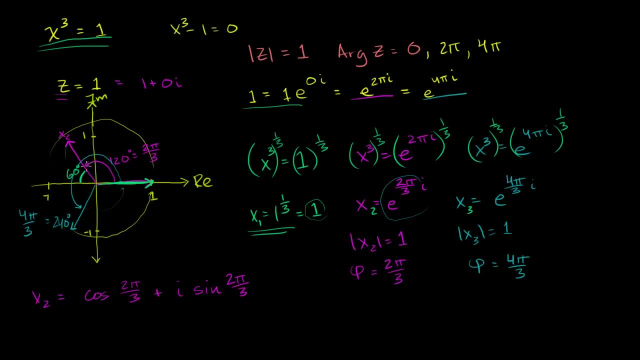 because this up here is 30 degrees and the hypotenuse or the length is 1, then this over here is square root of 3 over 2.. And at this distance right over here is negative 1 half. So x2 is going to be equal to cosine of 2 pi over 3. 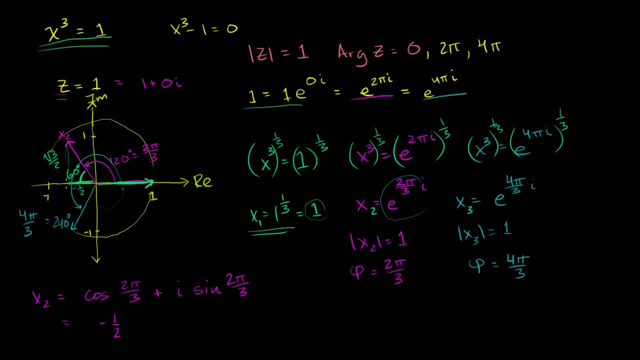 is negative 1 half. Did I do that right? Yep, Negative 1 half plus i times sine of 2 pi over 3.. That's this height over here which is square root of 3 over 2i, So that's x2.. 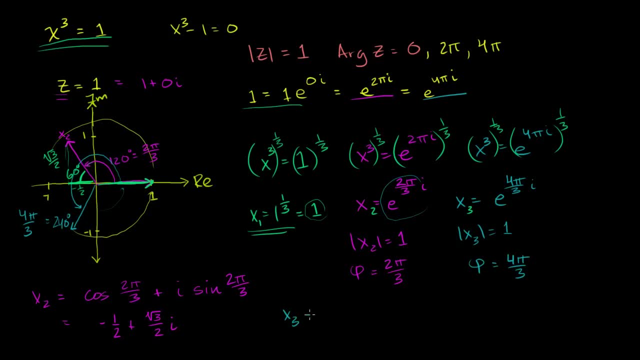 And we can do the exact same thing with x3.. x3 is going to be equal to its x value, Or I should say its real value is going to be the exact same thing. It's going to be negative 1, half, And then its imaginary value. so this angle right over here. 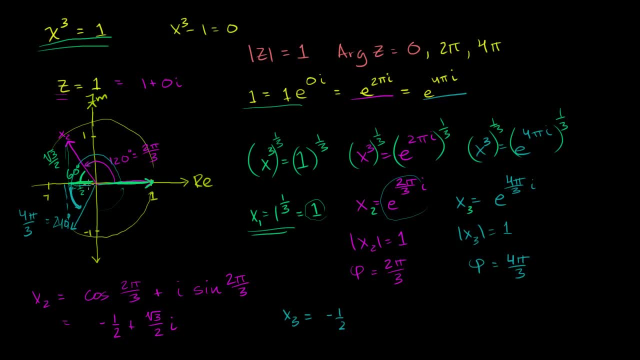 is going to be negative 1 half, So that's x2.. And this angle right over here, this just from the negative real axis down to the vector, is going to be negative 60 degrees. So this height right over here is going to be negative square root of 3 over 2.. 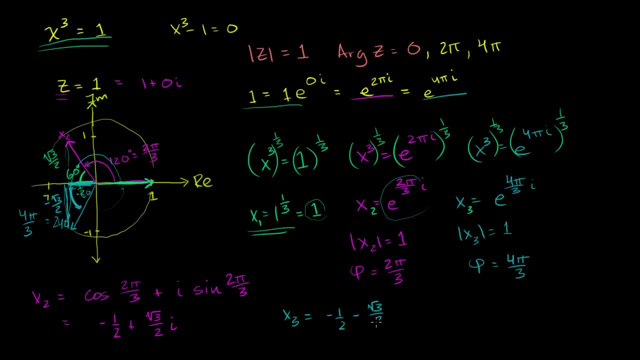 So it's negative 1 half minus the square root of 3 over 2i. So, using this technique, we were able to find the three complex roots of 1.. This is one of them, This is another one And, of course, 1 is one of them. 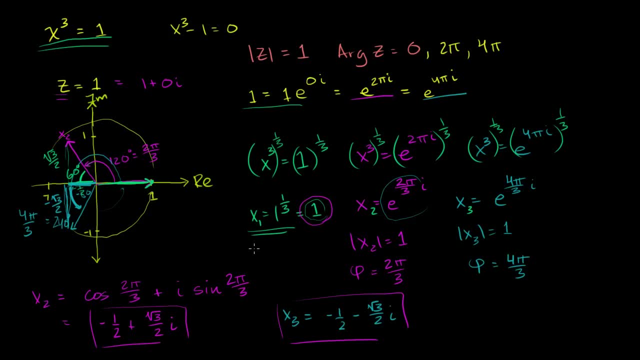 1 is one of them as well. Where did we do that? 1 is one of them as well, And you could use this exact same technique If we were finding the fourth roots. we would take the 2 pi radians or the 360 degrees. 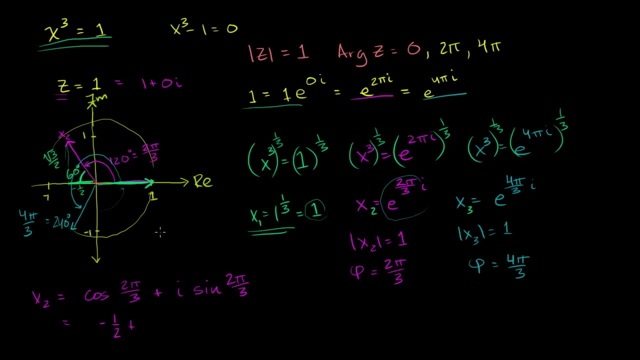 Did I do that right? Negative 1 half Plus i times sine of 2 pi over 3.. That's this height over here which is square root of 3 over 2i, So that's x2.. And we can do the exact same thing with x3.. 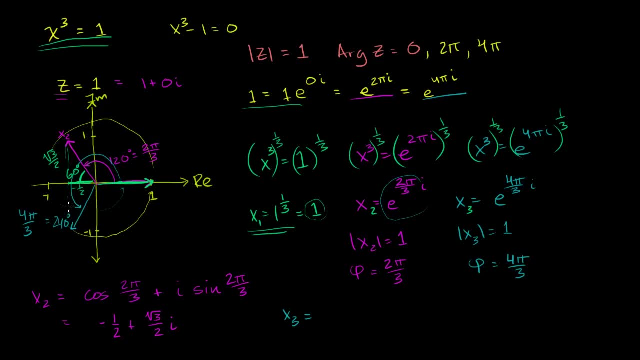 x3 is going to be equal to its x value, Or I should say its real value is going to be the exact same thing. It's going to be negative 1 half, And then its imaginary value. So this angle right over here, this just. 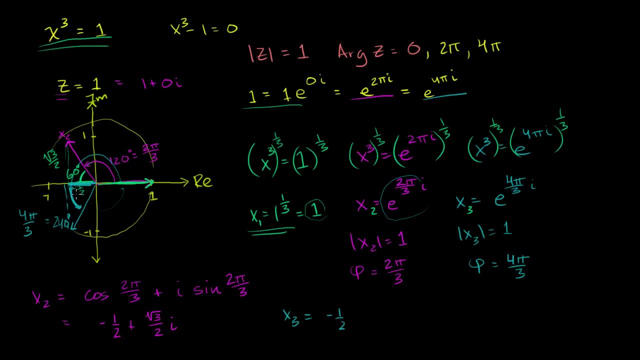 from the negative real axis down to the vector is going to be negative 60 degrees. So this height right over here is going to be negative square root of 3 over 2.. So it's negative 1 half minus the square root of 3 over 2i. 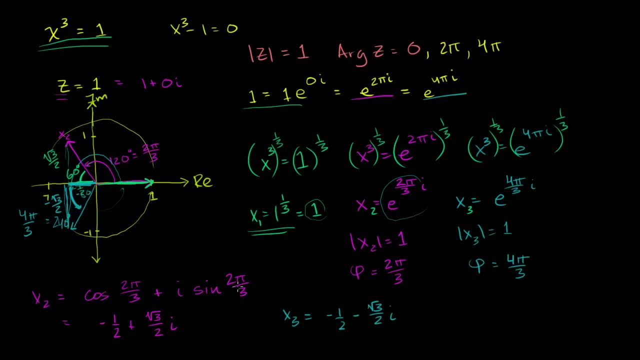 So, using this technique, we were able to find the three complex roots of 1.. This is one of them, This is another one And, of course, 1. Is one of them as well. Where did we do that? 1 is one of them as well. 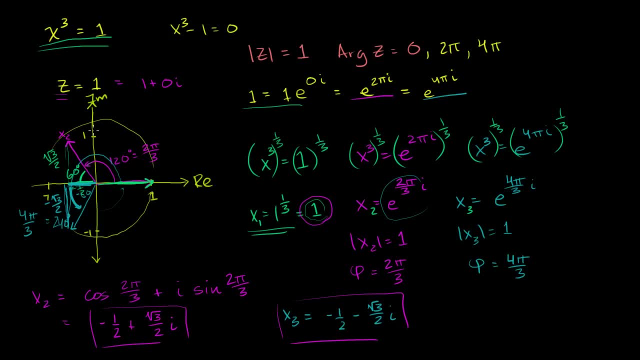 And you could use this exact same technique If we were finding the fourth roots. we would take the 2 pi radians, or the 360 degrees, and divide it into 4. And so it would actually be this. It would be i. 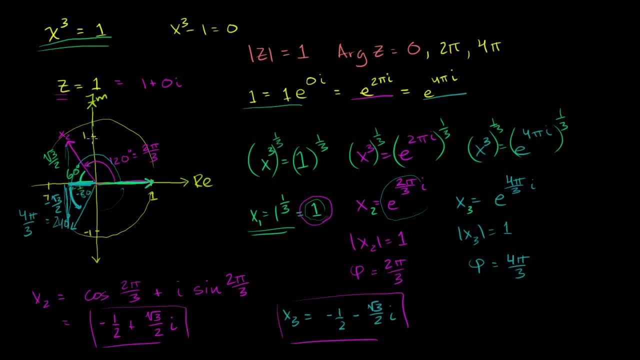 It would be negative 1.. It would be negative i. And we know: if you take i to the fourth, you get 1.. If you take negative i to the fourth, you get 1.. And if you take negative 1 to the fourth, you get 1.. 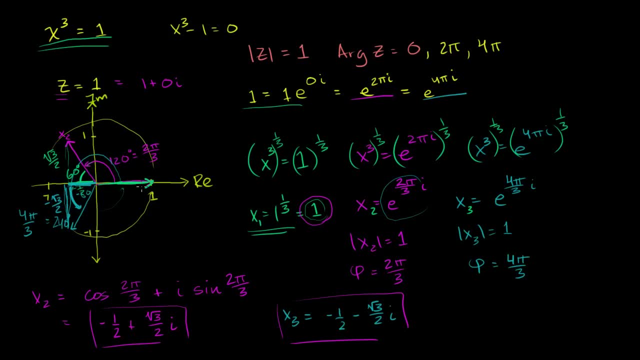 And if you take 1 to the fourth, you get 1.. And so you could do this. You could find the eighth roots of 1 using this technique. Now, the other question that might be popping in your brain is: why did I stop at e to the 4 pi i? 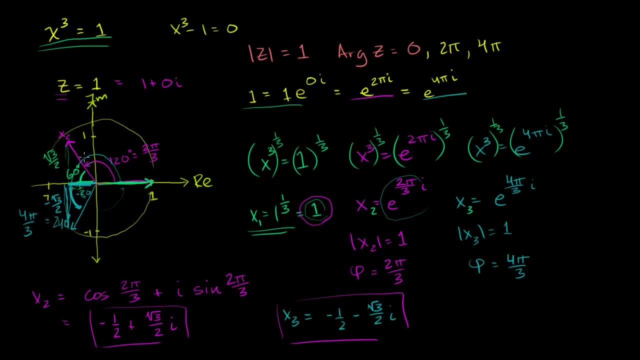 and divide it into 4.. And so it would actually be this. It would be i. It would be negative 1.. It would be negative i. And we know, if you take i to the fourth, you get 1.. If you take negative i to the fourth, you get 1.. 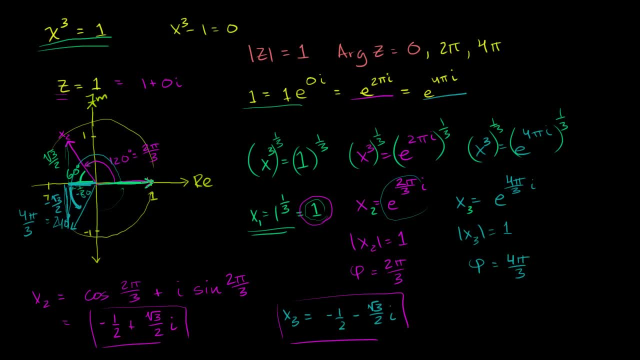 And if you take negative 1 to the fourth, you get 1.. And if you take 1 to the fourth, you get 1.. And so you could do this. You could find the eighth roots of 1 using this technique. 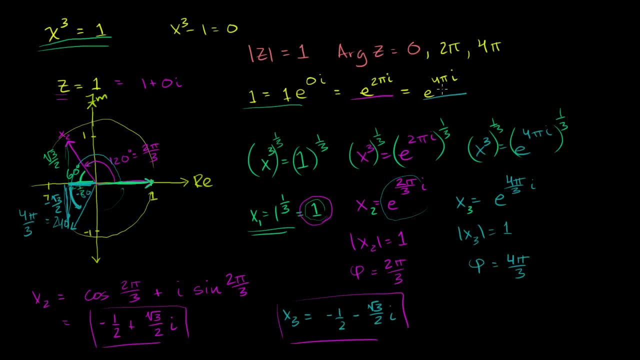 The other question that might be popping in your brain is: why did I stop at e to the 4 pi i? Why didn't I go on and say: well, this is equal to e to the 6 pi i and look for another root? 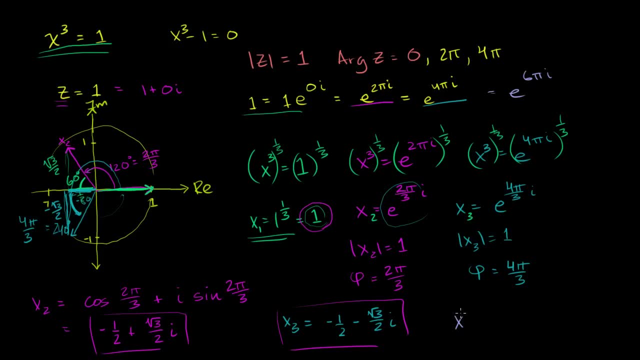 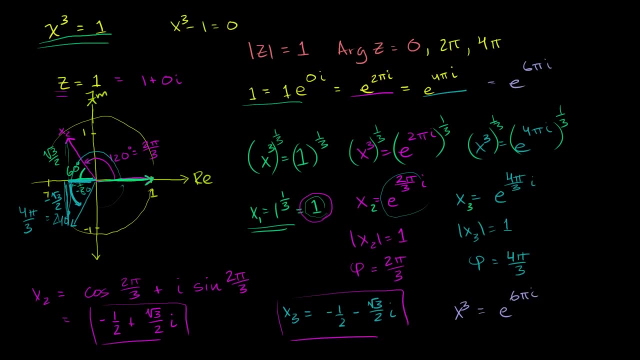 And so if I did that, if I said x to the third- let's say I wanted to find a fourth root here. maybe x to the third is equal to e to the 6 pi i- And I take both sides of this equation- to the 1 third power. 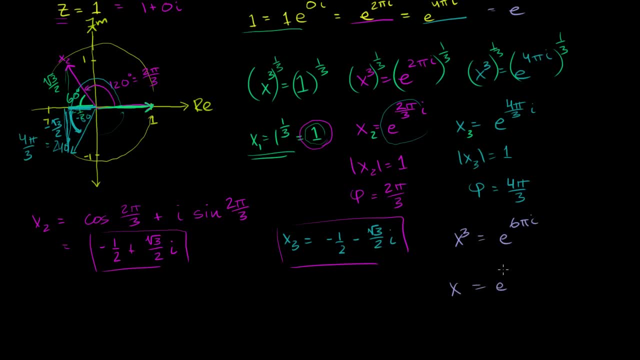 So I'd get x is equal to taking this to the 1 third. I'd get e to the 2 pi. I'd get e to the 2 pi. i. Well, what's e to the 2 pi? i e to the 2 pi. i will just get us back to 1.. 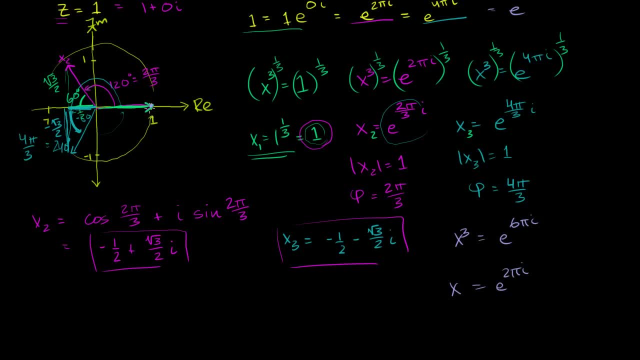 So when I added 2 pi again, it just gets us back to this root again. And if I took e to the 6 pi, if I took e to the 8 pi, I would get this root again. So you're going to get only three roots. 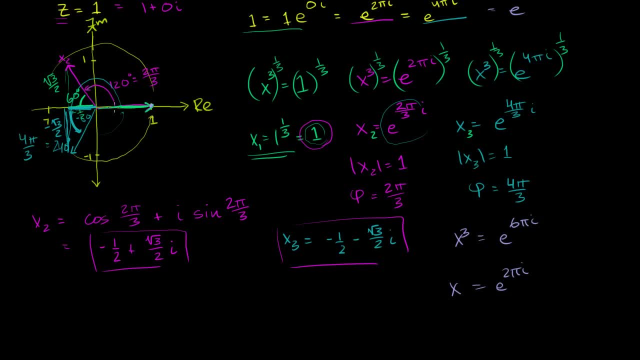 if you're finding the third roots of something. Anything beyond that, it just becomes redundant. 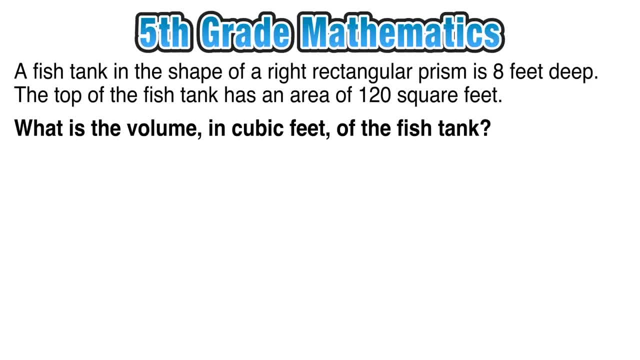 What's up and welcome back fifth graders. Thank you for joining me on this problem. Let's go ahead and dive right into it, No pun intended. In this case we have a fish tank in the shape of a right rectangular prism that is eight feet deep and the top of the fish tank has 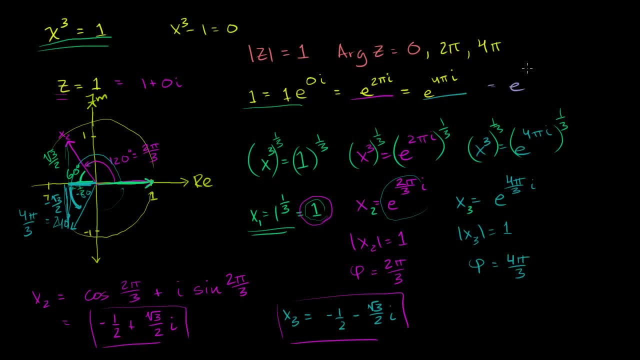 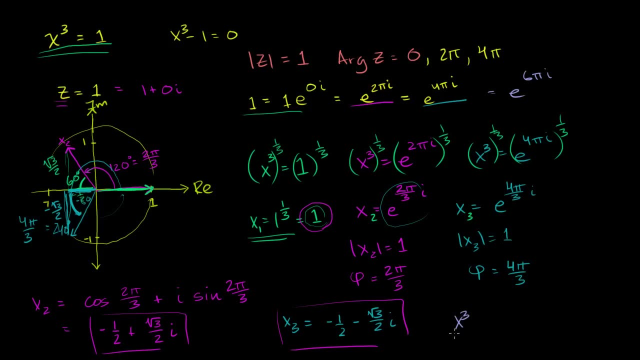 Why didn't I go on and say, well, this is equal to e to the 6, pi i, and look for another root? And so if I did that, if I said x to the third, let's say I wanted to find a fourth root here, maybe. 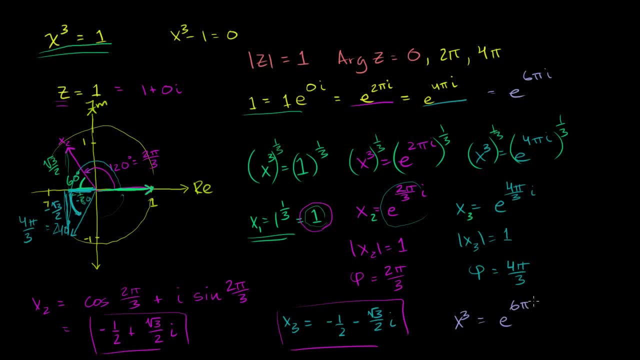 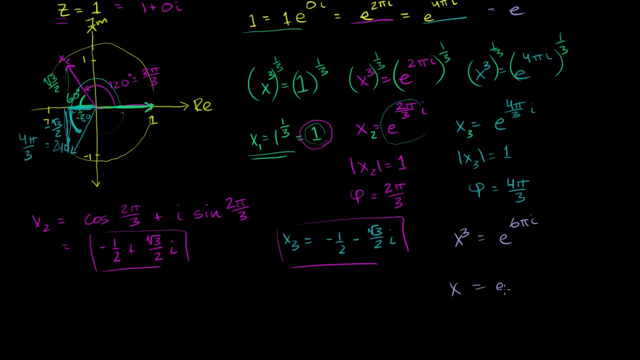 x to the third is equal to e to the 6 pi. i And I take both sides of this equation to the 1 third power, So I'd get x is equal to taking this to the 1 third. I'd get e to the 2 pi.